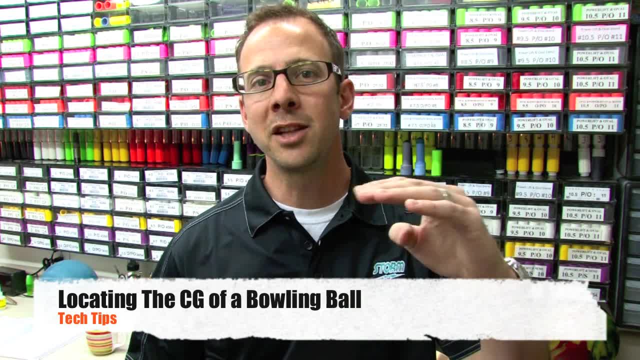 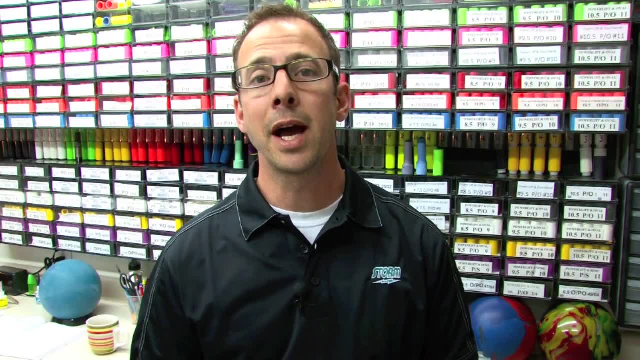 extended it up to the surface. that's where you get the eye of the storm. That's where the center of gravity is- on the surface of the ball, the marking- while the true CG actually lies below the surface. Now you can locate the center of gravity of any bowling ball. We're going to 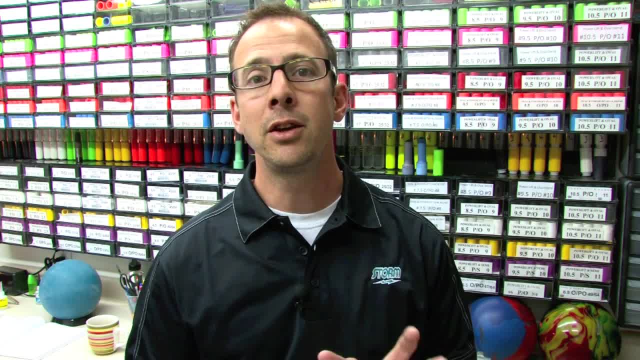 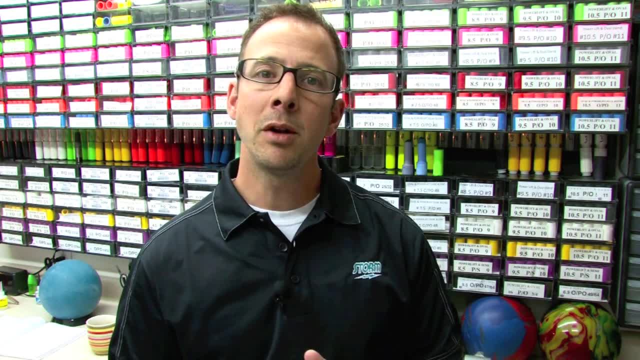 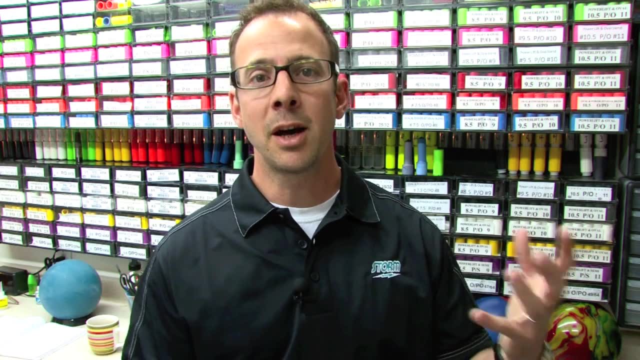 demonstrate it today on a drilled bowling ball, but realize that you can also use the same method to locate the center of gravity of an undrilled bowling ball or a plugged bowling ball. Now, this is important because when you remove the weight with the drilling holes, you're actually removing mass at an unequal level. So when you replace 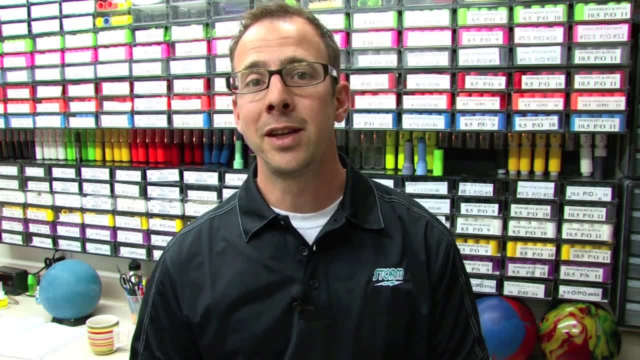 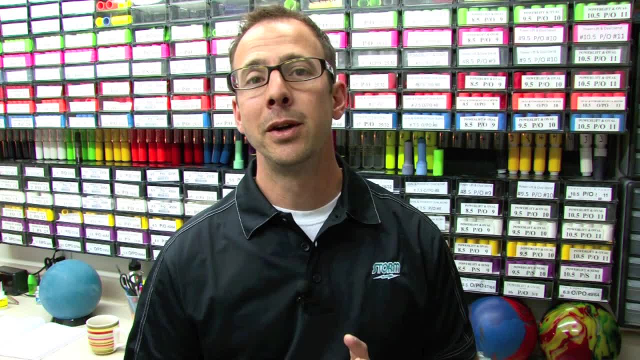 that with ball plug, you're going to move where the true center of gravity is actually located. It's no longer going to be where it was when it was undrilled, So that's important to remember. Second thing that's important to remember is that we still have regulations from the 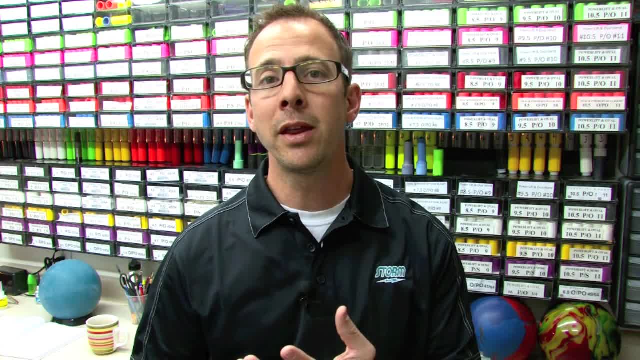 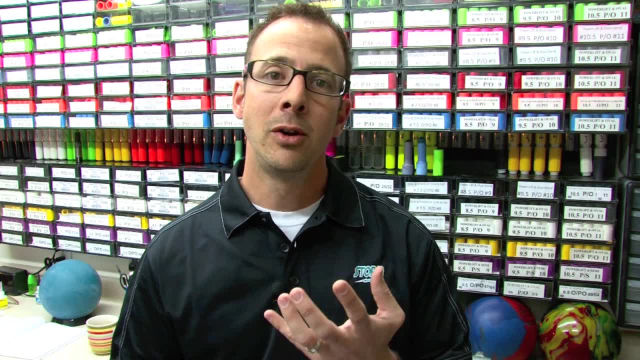 USBC on the static weight of our ball. So you can't have more than an ounce of positive weight or more than an ounce of thumb, for example. so you still have to know where that's located and make sure that the ball still weighs up and meets those specific weights. 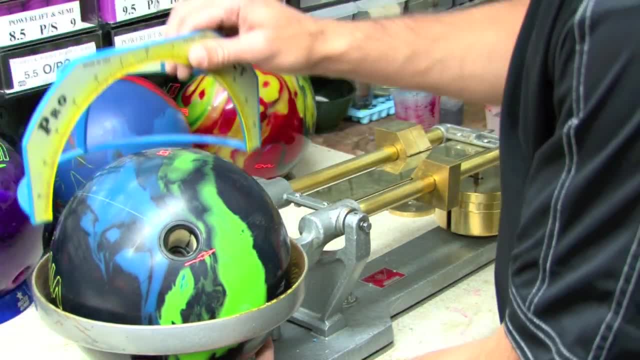 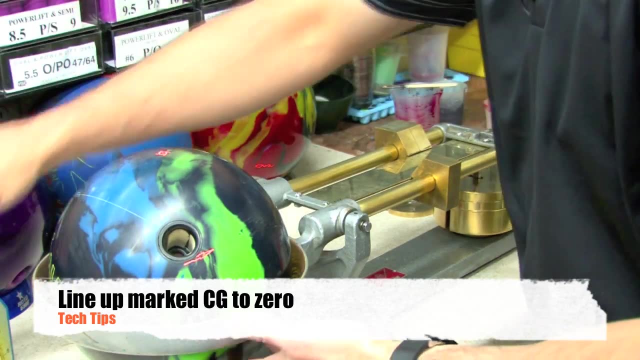 All right. so the first thing we're going to do is we're going to place that bowling ball in the cradle here and we're going to try and line up the marked center of gravity right at zero on our Proceq. So we'll take that off, we'll adjust the back beam, try and get it so it levels out making. 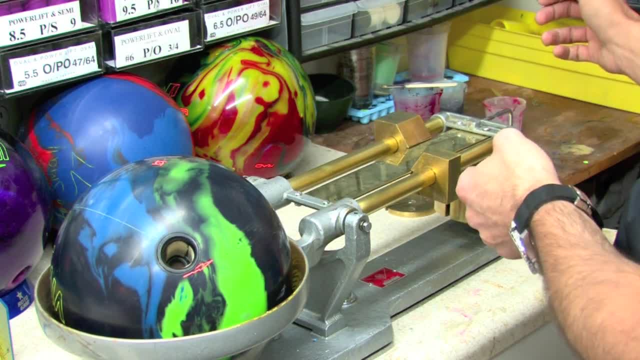 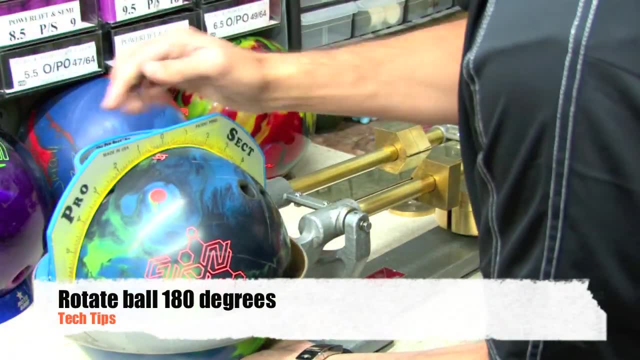 sure that our front beam is already set at zero, which it is Okay, so we're looking pretty good. Now we're going to rotate it 180 degrees Again. put your Proceq back on. We're going to rotate 180. 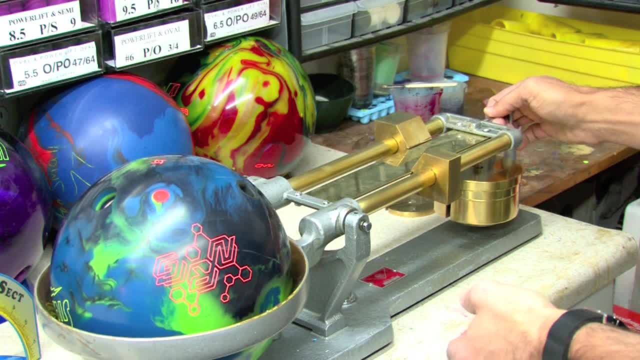 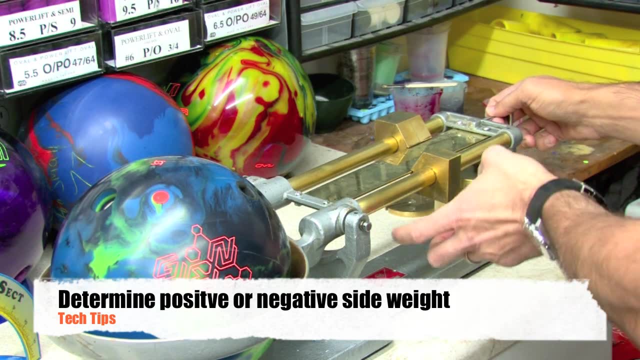 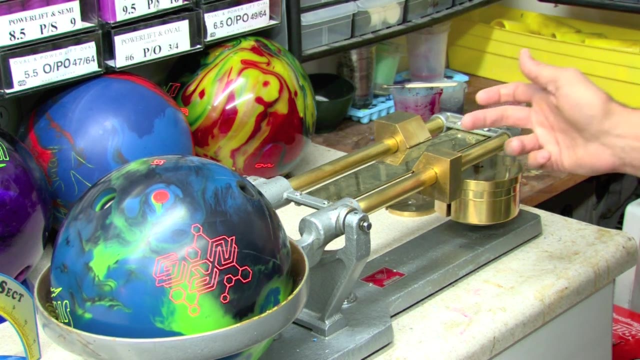 degrees, and we're going to try and line that up. Now. we're going to see how much positive or negative side weight we have from that point. Okay, we've got a little bit of positive weight there. We're going to see exactly what it is. It weighs out about a quarter, So what? 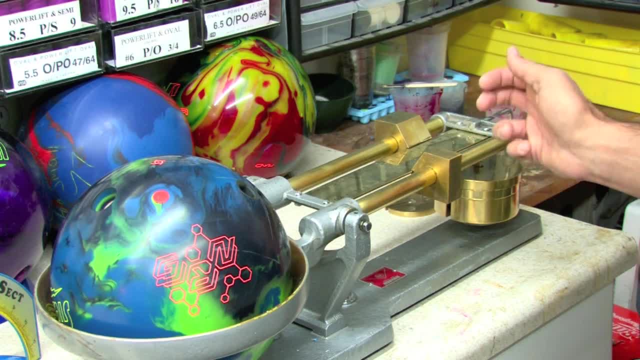 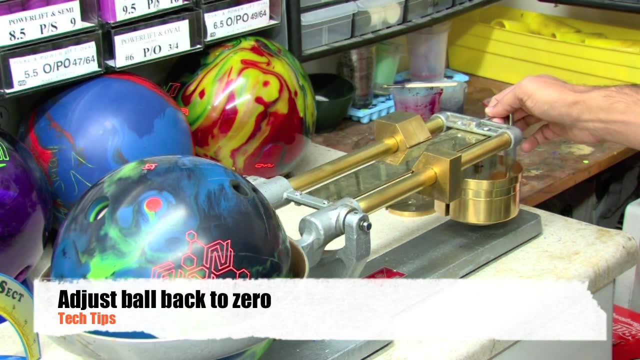 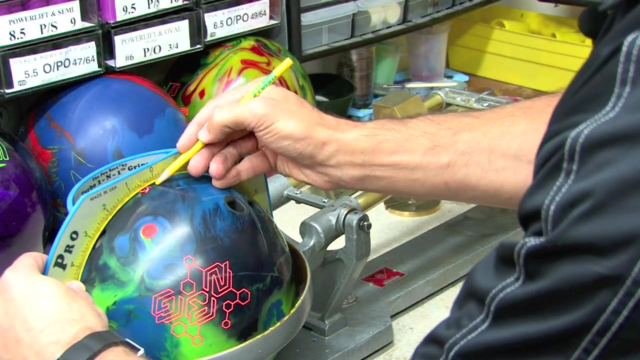 we do is we take half the difference, we move that balance back to an eighth and now we're going to adjust the ball and try and get this to balance and be back at zero again. Looks like a pretty good shot right there, So we'll put our Proceq back on mark the zero point. 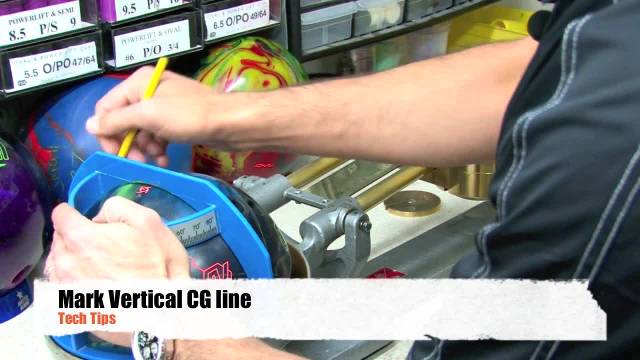 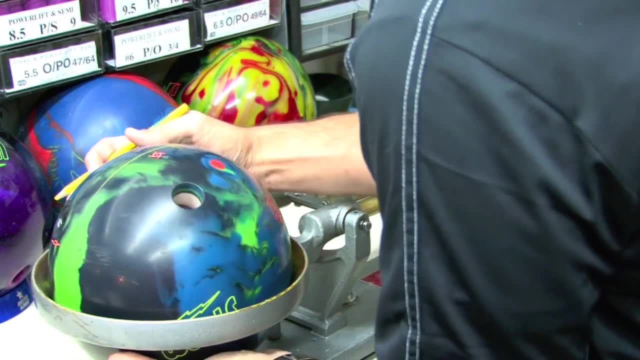 and then we'll go ahead and mark our line. This is our what I would call a vertical line here, where the center of gravity is going to be somewhere along this line. Now we've got to figure out exactly where, along that line, the center of gravity is, So we're going to do the